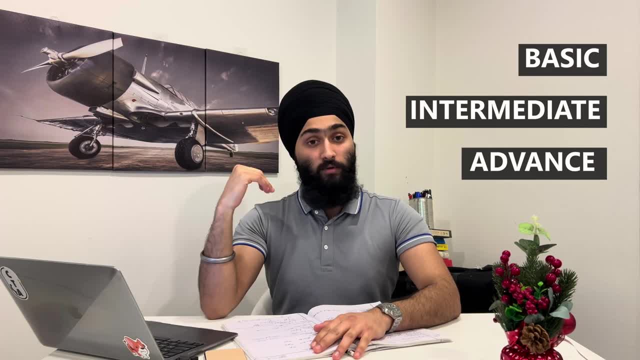 categorized this video based on three level of depths, For example. first level of depth is for the people, those who are like me, those who love to study virtually but they cannot go into technicalities. Second level is for the people, those who are interested in technicalities. They 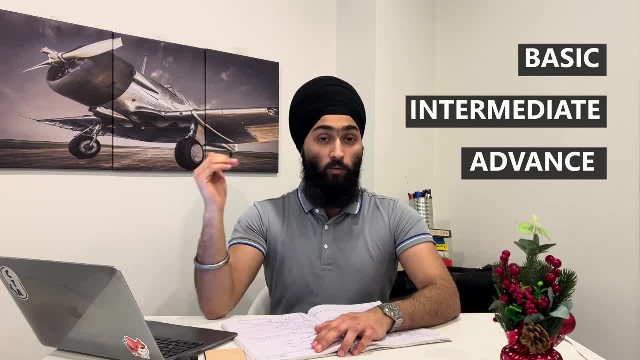 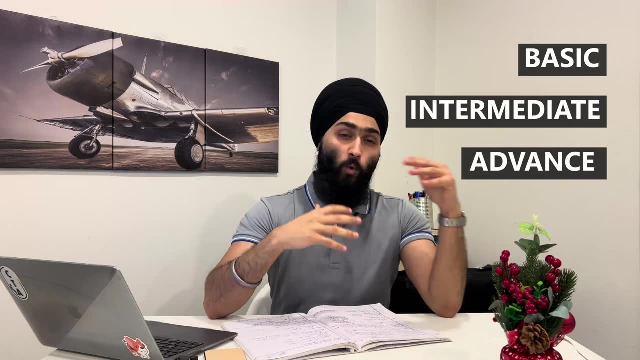 want to solve numericals, how everything works, and they want to solve equations. The third level is for the people, those who want to research in this industry and they want to learn more about the technicalities. So these are going to be three level of depths. These resources are categorized. 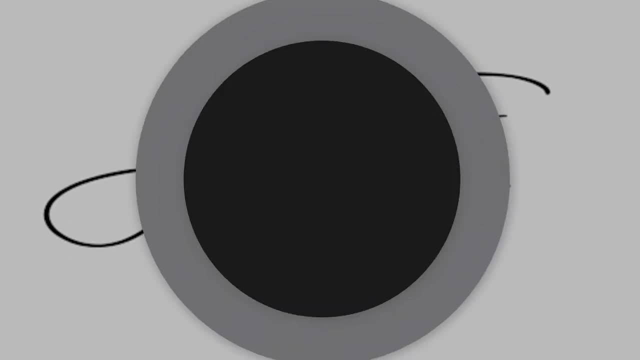 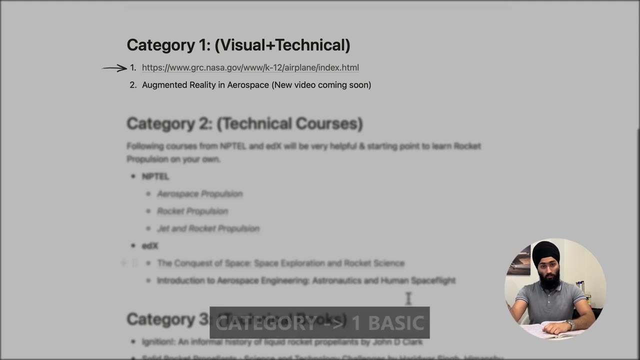 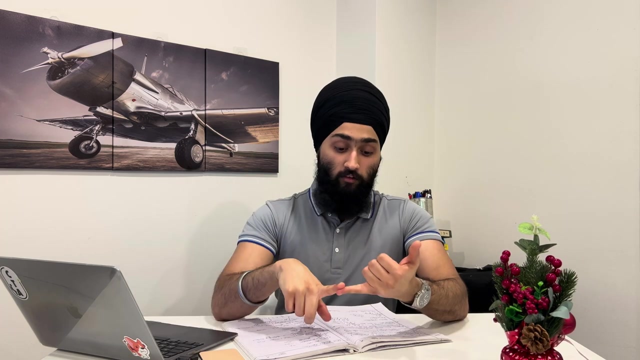 into. So let's talk about the first resource in the first category, that is, the official webinar. So let's talk about the first resource in the first category, that is, the official webinar, Because they have included simulations, then they have many of the activities and it is so visually. 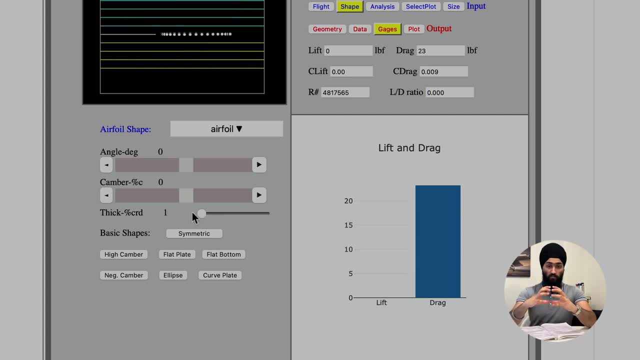 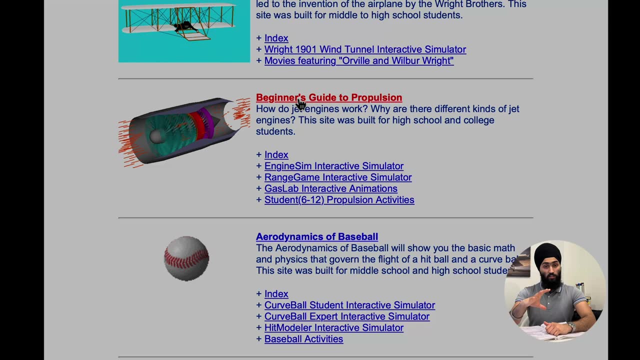 appealing. for example, they have included various gives in that as well. I am talking about airplanes, talking about ballistics also. a jet engine works and it's a great resource even nowadays. so these resources are my favorites at all because they have included simulations. then they have many. 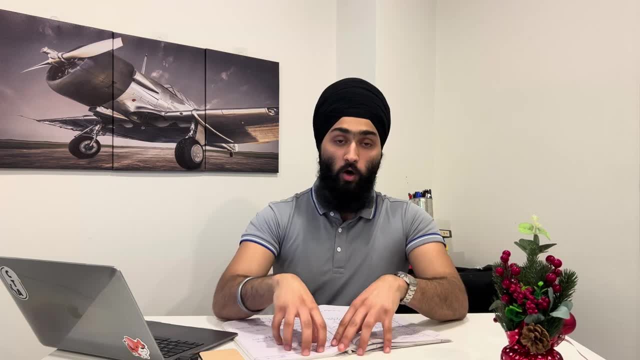 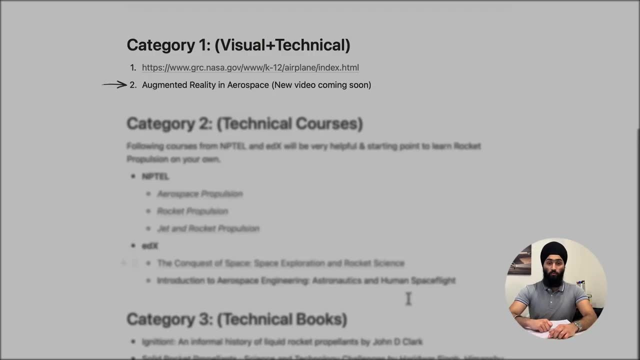 go to that website just to pass my time, because whenever i'm hooked onto their website i do learn a lot, many new things. jumping onto the second resource, that is, learning through augmented reality. so if you are a tech guy, you know about augmented reality. if not, do not worry. my next, 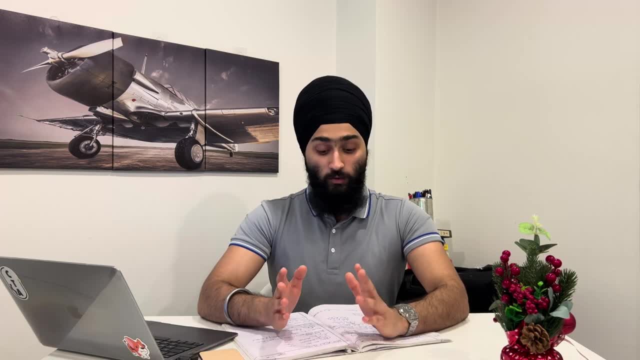 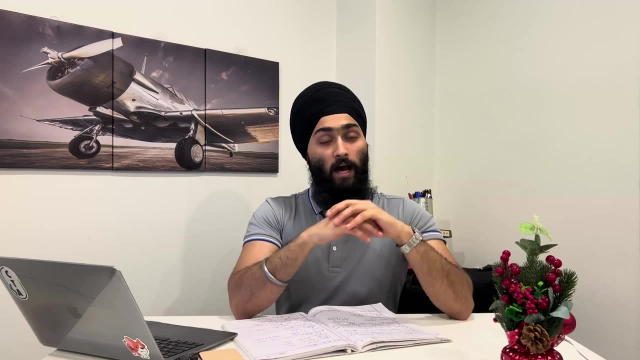 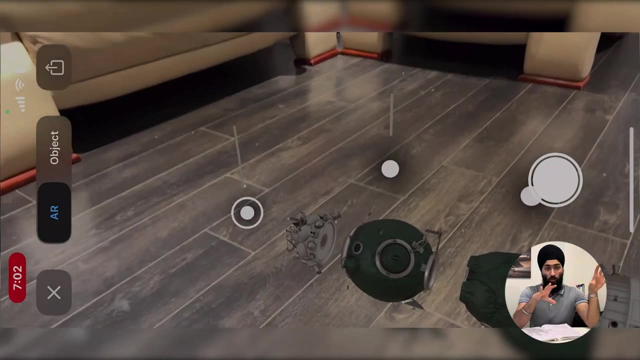 video is going to be about augmented reality in aerospace. so this is also my best category, because i love to learn virtually. so whenever i want to learn something new, i just go to a website and i just turn on my iphone's camera and i just learn more about what is command module. 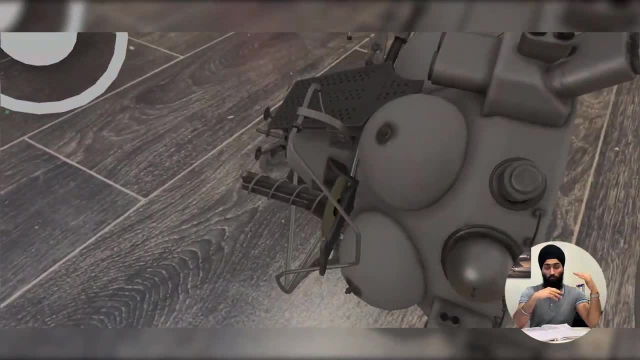 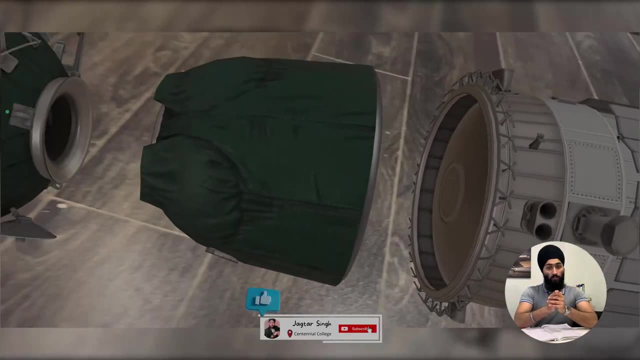 what is lunar module? what is? what are the different things about spacecraft? so everything like that. i love to learn through augmented reality. so if you want to know more about this video, subscribe to my channel, because this is going to be my next video. let's jump to the second category, that is, 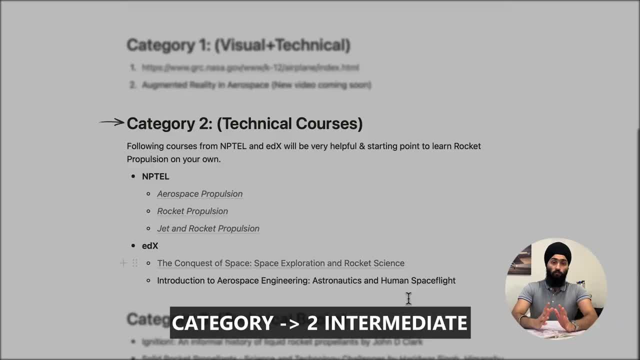 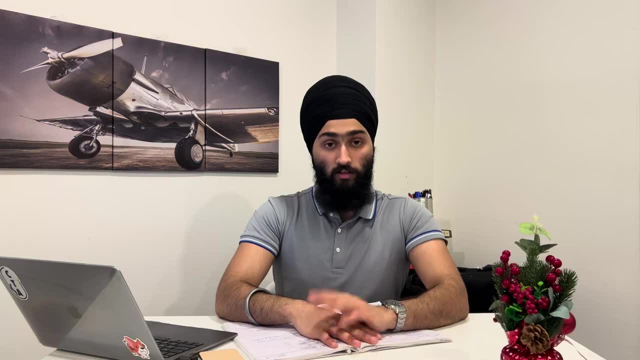 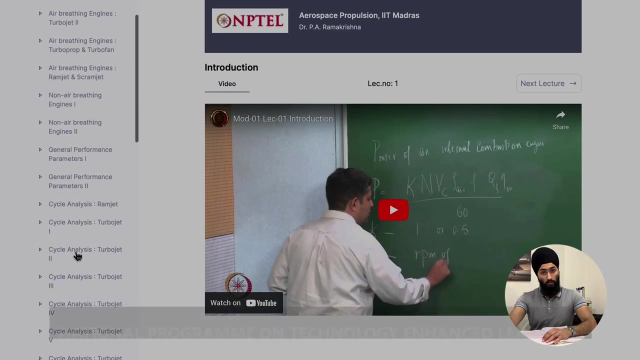 for the person, those who love technicalities. so let's talk about the various courses which are available out there online for free of cost, which you can do all by yourself. so there are two resources out there. so first resource in second category is nptel initiative, that stands for national program on technology. 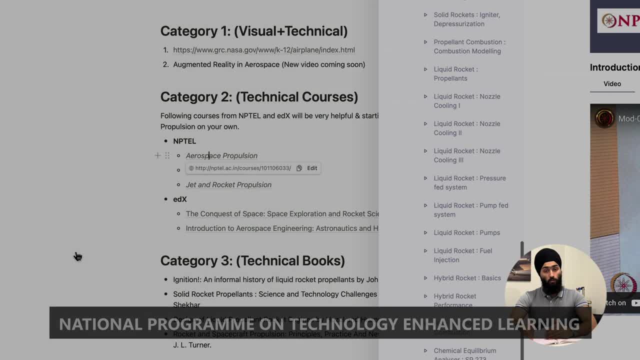 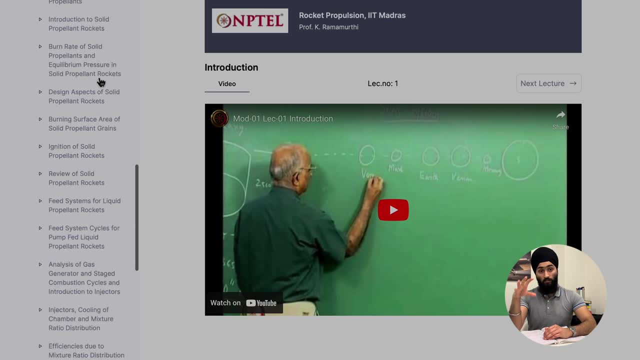 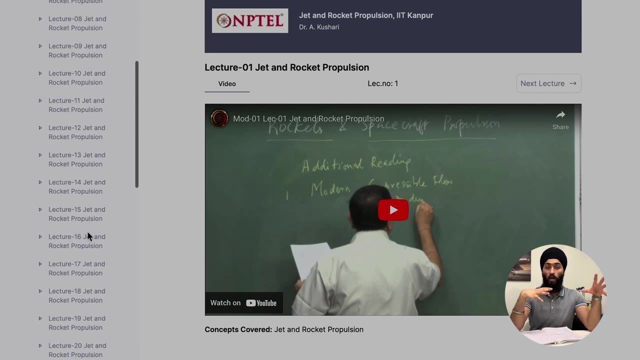 enhanced learning. so this initiative is by indian institute of technology and iisc bangalore. they have created a course specifically for rocket propulsion. enthusiast, those professors are ide professors, those who are teaching you how things work, how rockets work, how everything in aerospace engineering works. so basically, i have 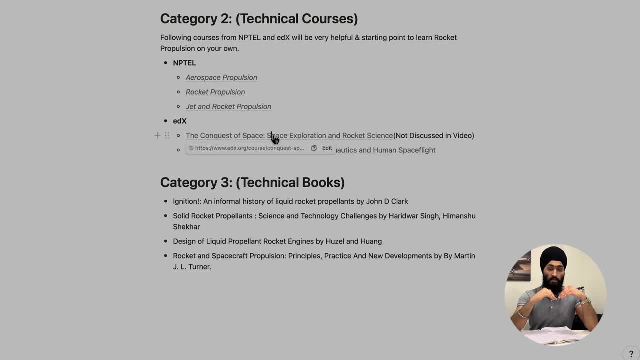 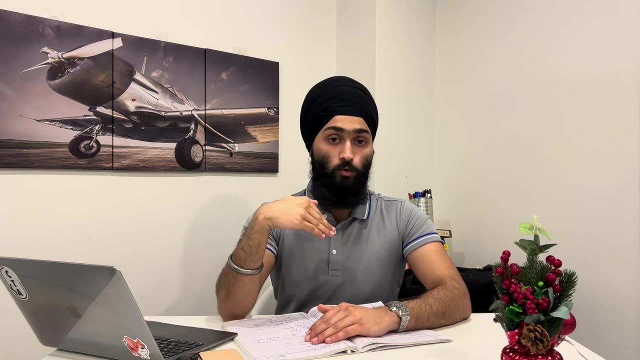 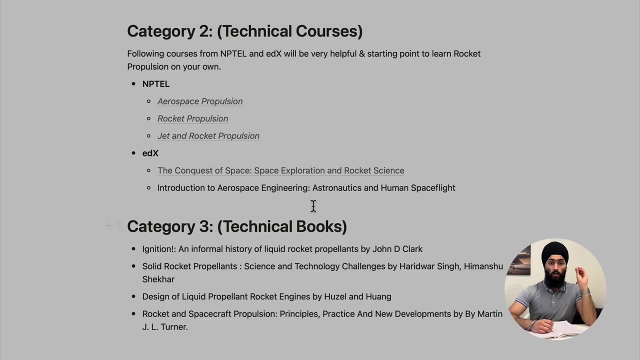 personally done their course. there are three major segments, major courses out there. i just put a document in the description below so that you can actually go to that link and access those courses for free. second resource is the online courses on edx. so there are two major aerospace engineering. 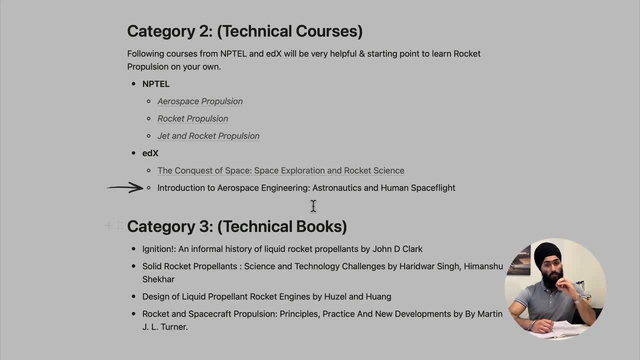 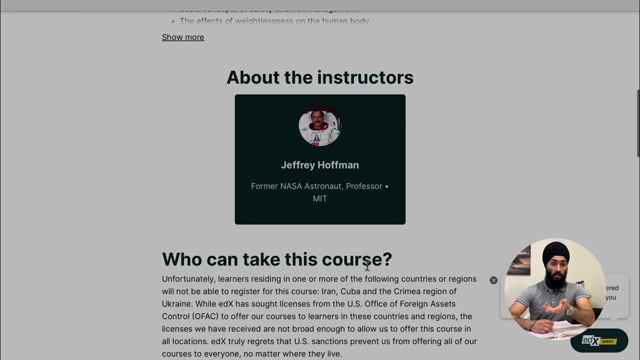 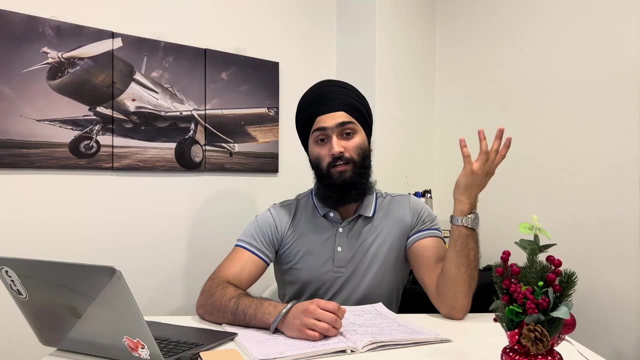 courses which are out there. first one is introduction to aerospace engineering. that is Coleon. so that's the first one, that's the second one and the last one is humans of the universe. so this is the name of the course that i have done. it is actually done by jeffrey hoffman, astronaut. so 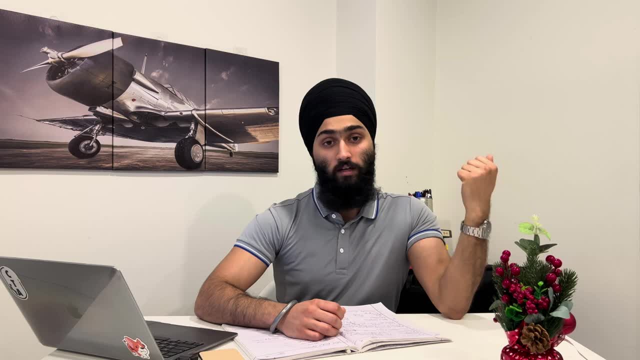 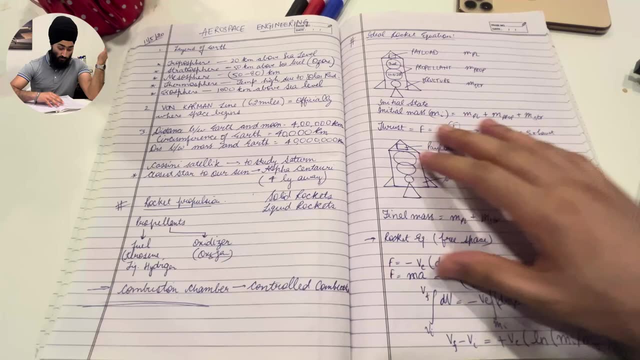 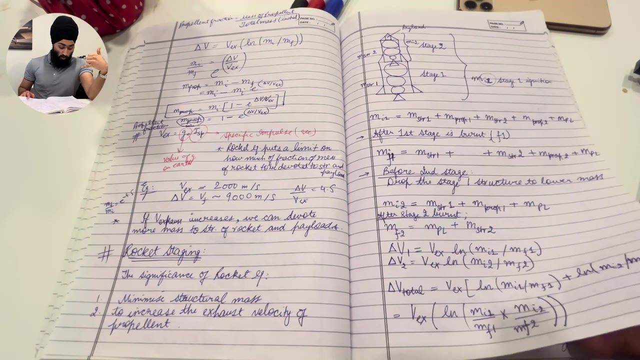 if you are aerospace enthusiast, you know that guy because, to be honest, he was idle to me- so to learn from such a professor- he's a professor at MIT, so to learn from that astronaut, it was amazing. so i have done this course in the lockdown. so these, these are actually the notes which i have made, so in this. in this course, they have literally talked about rocket staging. when, when i wrote this, i think it was in the first period of the year that i wrote this. so when i write this in the course, when i wrote this, it is a simple thing, because this is not just a video. you can do it. 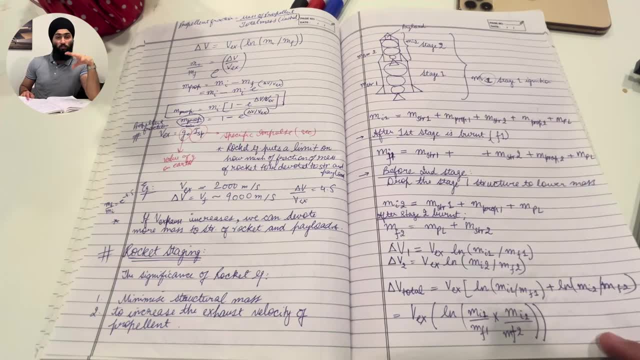 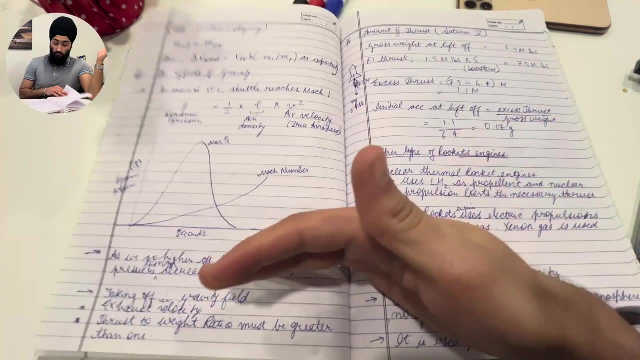 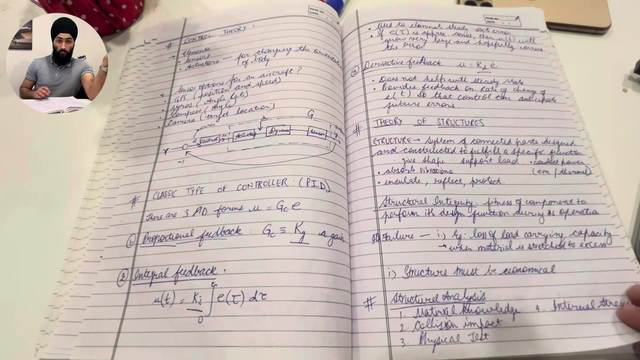 when, when the rocket lifts off from the earth, what are the various stages it goes through- stage one, stage two- and how to calculate rocket propulsion and rocket equations. they have also talked about what are the various types of rocket engines, how to calculate the amount of thrust by all the by. 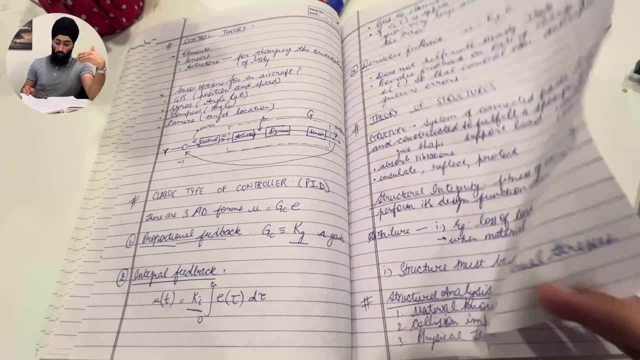 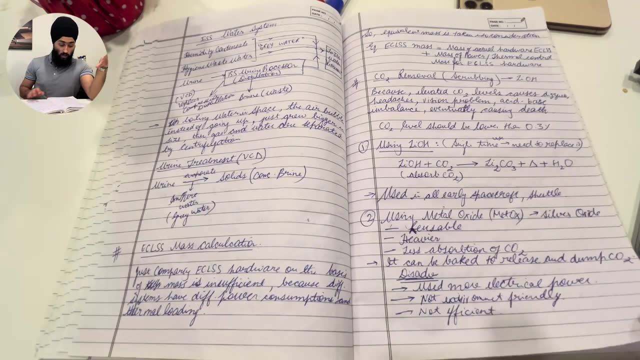 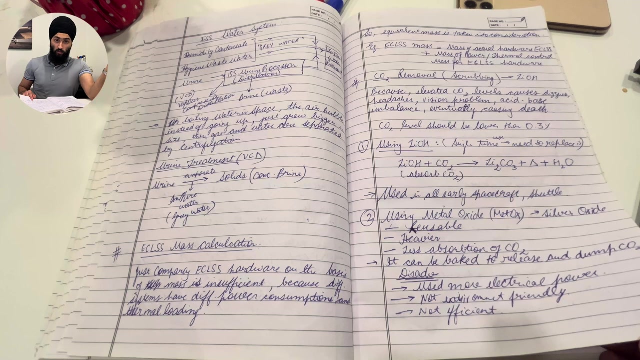 giving up all the examples. so they have talked about theory of structures, what is eclss and how they maintain the temperature of the cabin. so water systems and how they do the rendezvous that is a concept in astronautics. and then they also talk about the circular orbits, basically.